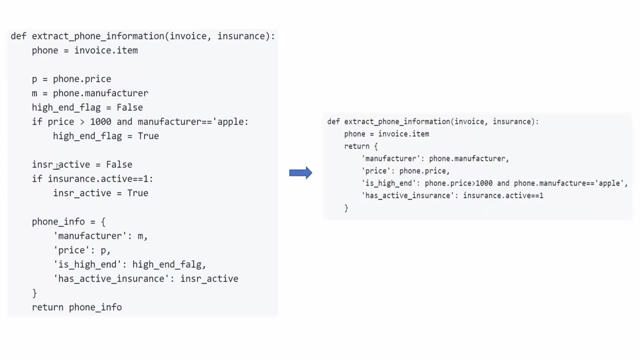 so, if you think about it, this p? m is iron insr underscore active. all these are unnecessary variables which can be avoided by writing this very, very compact code. so this code is not only compact, it's removing all unnecessary variables. i have seen so many codes uh during my 15 years of. 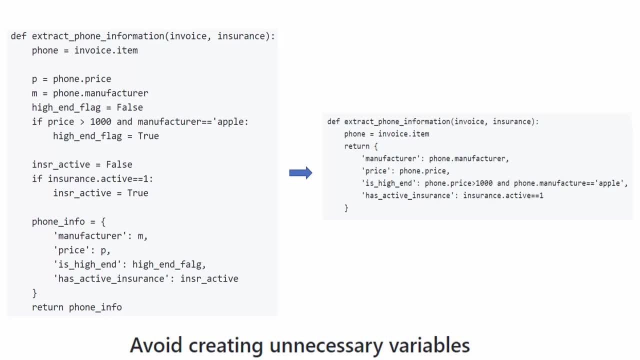 software programming experience. when i'm doing code review of other people's code, they end up using a lot of unnecessary variables. i mean, i was also doing that, but now i have gotten into a habit of writing a compact code. you use a variable only if it is used at multiple places, for example here: 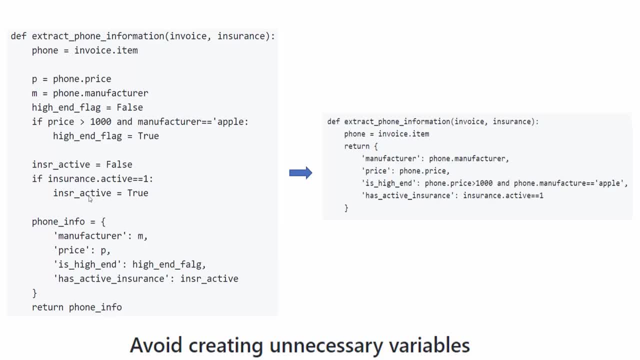 you use p as a phone price and then p you are directly using here, right? so p is not used anywhere else. so why don't you write phoneprice directly here? also, phone info structure is created and then returned but then not used at multiple places. so why don't you just create that on fly in a return statement? 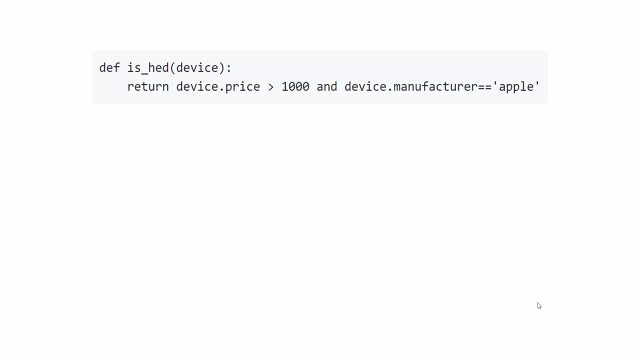 think about what is wrong with this code again. put a pause and just do some thinking on what could be bad with this code. let's say you are right. you have this function in your big code base where multiple people are working and a new person joins your team and he's looking at this code and he'll be like: is hed, what is actually what the heck is? 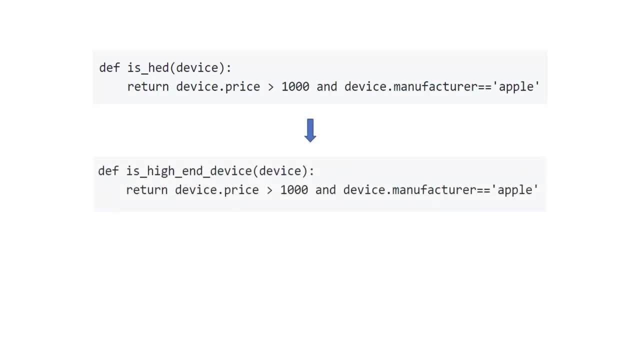 right if you use a full name is high end device. so the idea here is to avoid abbreviation as much as you can. abbreviations are biggest killer or and they cause a lot of confusion, even elon musk at tesla. he issued guidelines to all his employees that do not use abbreviation. 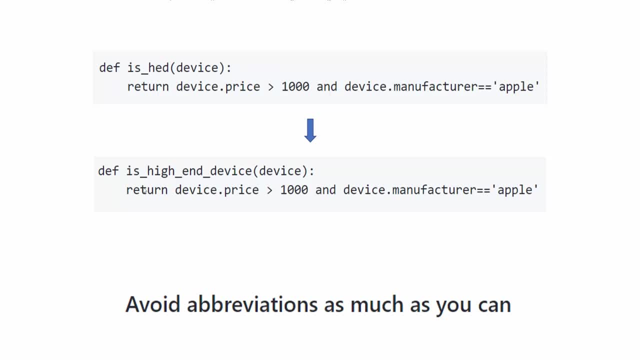 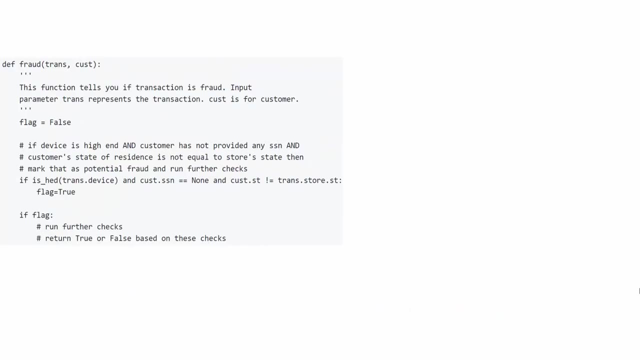 until absolutely necessary. here your function name will be little longer. but so what? it's fine, you can have longer function name, it is perfectly okay. but this makes your code more readable and less confusion. okay, now, what's wrong with this code here? in this code we are using 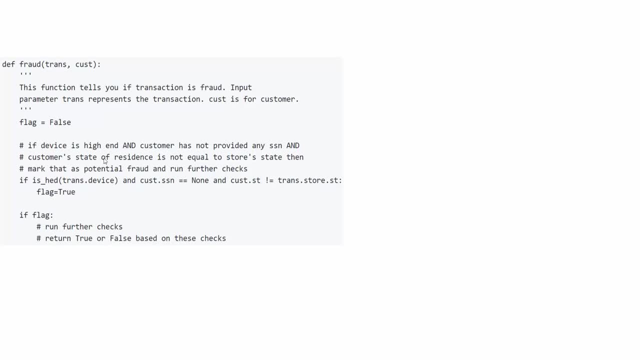 comments to describe what this code is doing, which is fine. but the biggest issue is with comments is that they get stale very easily. in a big code base, many programmers are working. a new programmer will come and that programmer will change this logic, but he or she will not update the comments and the comments become stale and confusing. 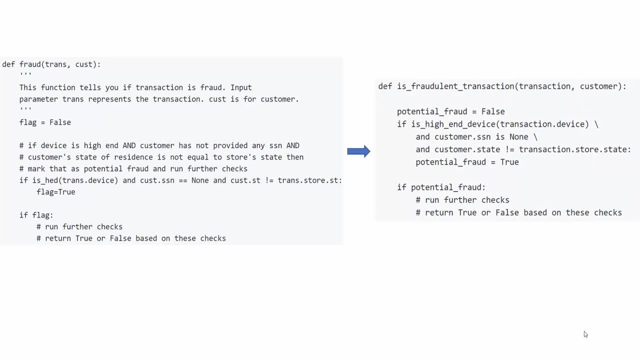 instead of using comments, how about we use descriptive function name and variables names to describe what we are trying to do? so in this code on the right hand side, i do not have any comments, but my function names are very, very clear and they describe the purpose clearly. for example: 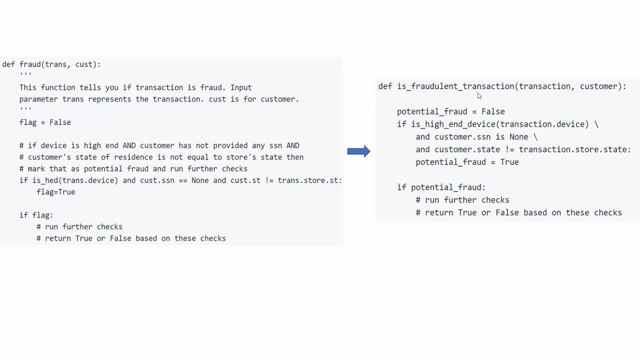 instead of saying fraud, i'm saying is fraudulent transaction. so if someone joins my team and he starts working on this code, the person will know that this function is trying to figure out if this transaction is fraudulent or not. similarly, here i'm using flag, but on the right hand side i'm not. 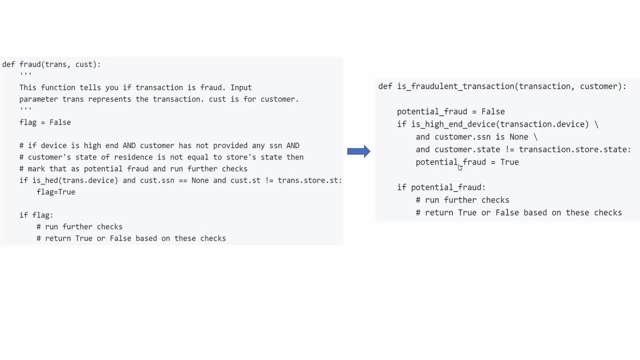 using that flag. i'm just saying potential fraud and when you read this variable, you immediately get an idea that if this variable is true, it means the fraud. is you potentially a fraud? so the guideline here is to use descriptive function and variable names or code comments. all right, now what is wrong with this code? this code is very intuitive, by the way. 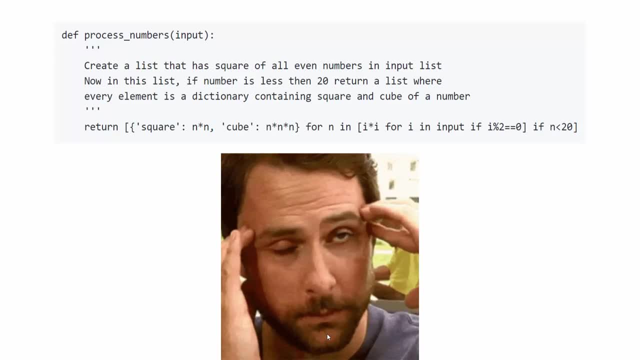 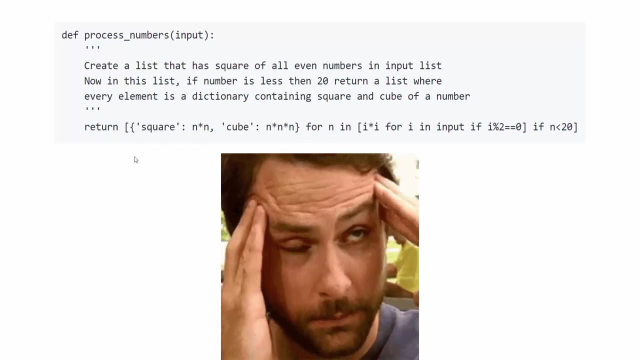 right, or is it giving you a headache? well, it will give headache to most of the programmers because there is this one line which is using some weird list comprehension, nested comprehensions in python, the. the guideline here is to use descriptive function and variable names over code comments. 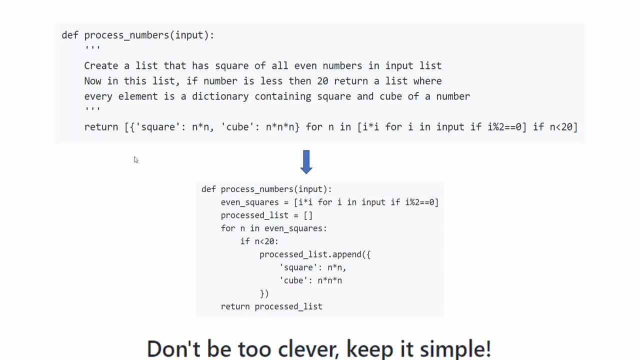 here is: don't be too clever, right? i have seen many programmers who just wants to prove that they are the smartest dude on the earth, you know, and they write all this crazy clever code. but do not write that clever code. keep it simple so that it is readable. sometimes the person who wrote even this. 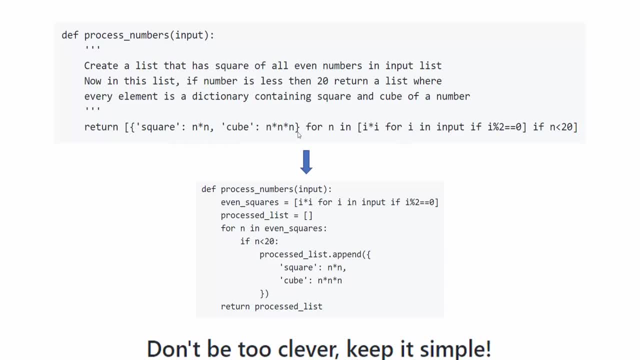 code after that, if that person refers to it after a month or so, the person himself will get confused. okay, so not only it's a problem for others, it could be a problem for others, but it could be a problem for the person who is writing this code. so write the code, which is simple now in python list comprehension. 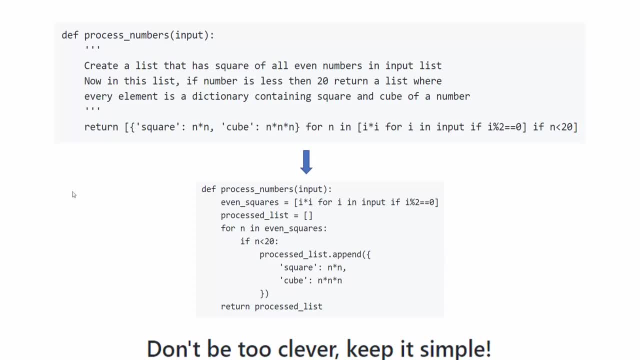 dictionary comprehensions gives you performance. but just think about like: is performance really needed? if i am running this code on a list with which has a size of only 20 elements, there is not practically any difference between the performance between these two cores. okay, when you are thinking. 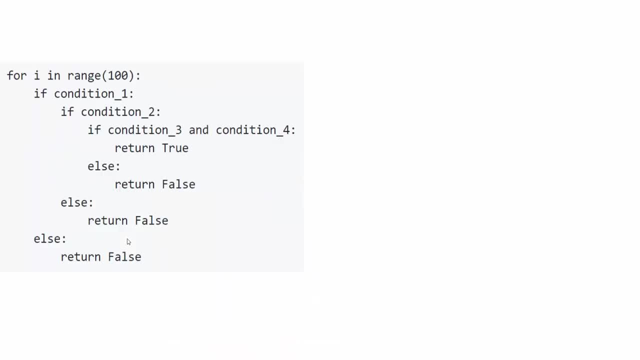 about performance. just be very practical, all right. now. what is wrong with this code? again, put a pause. try to write a better version of the same code. i am pretty sure you will be able to come up with a better version, all right. so, assuming that you have given your attempt, the answer here would be to avoid nesting as much as possible the same code. 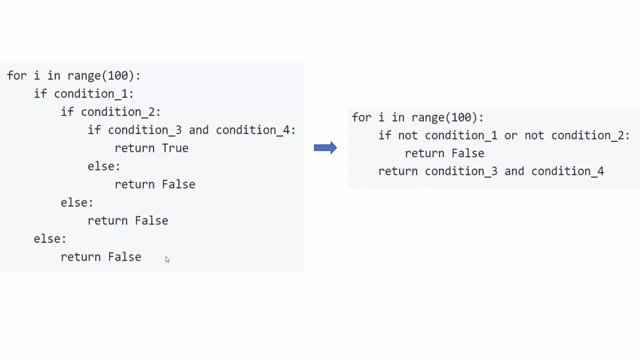 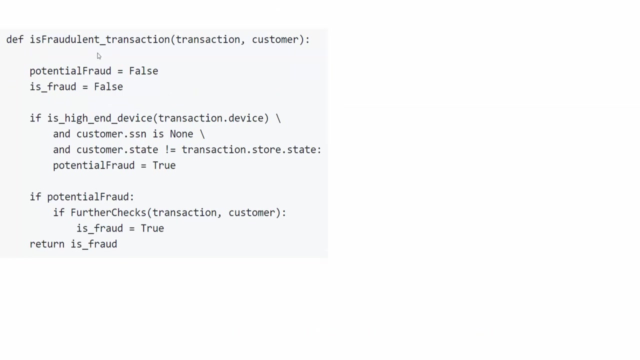 can be written in a compact way using three lines. so you see, instead of so many lines now, i have only three lines. so the guideline here is: too much nested code will kill code. okay, now what's wrong with this one? here we are using mix, a naming convention. uh, we are using a. 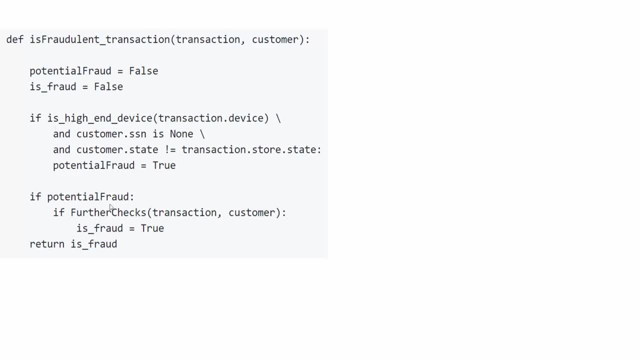 snake case convention here and uh also a camel case. so the guideline here is: whatever naming convention you're using, uh, just be consistent. so here i am using pap8 naming convention, but i'm being consistent throughout the code. so here you see, is fraudulent, is camel case, and then i'm 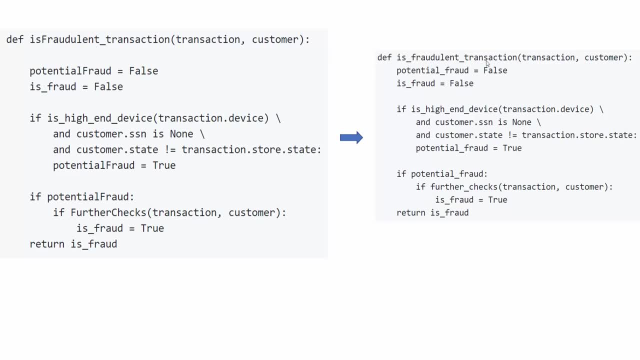 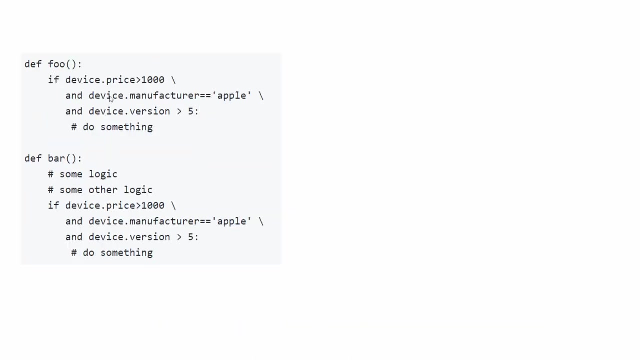 using underscore versus series is underscore, fraudulent underscore transaction. so everywhere i'm separating words by underscore and using a standard and consistent naming convention. i've seen many code bases where they use this mixed naming convention and it makes your code look really horrible. all right, how about this code? so i have foo and bar and i have this if condition. 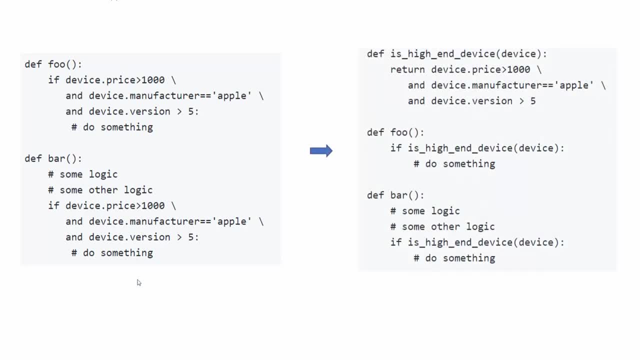 being repeated two times. we take this condition in a function and make a function out of it and use that function in foo and bar. so not only you are avoiding a duplication now, tomorrow, if someone has to change this condition in the left hand side, he has to modify multiple function on right hand side. you just 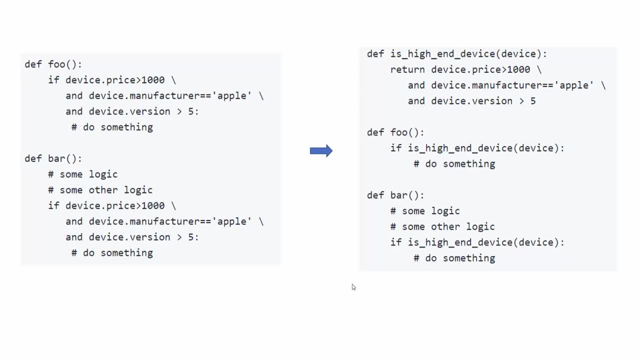 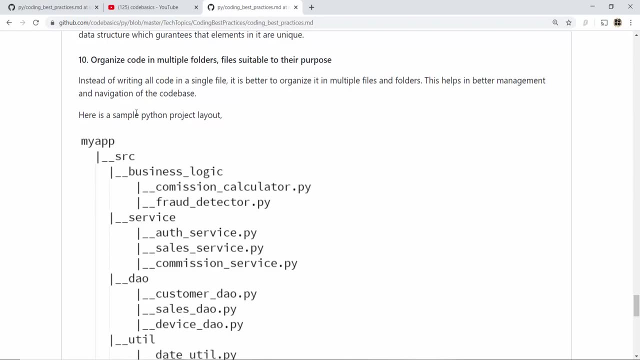 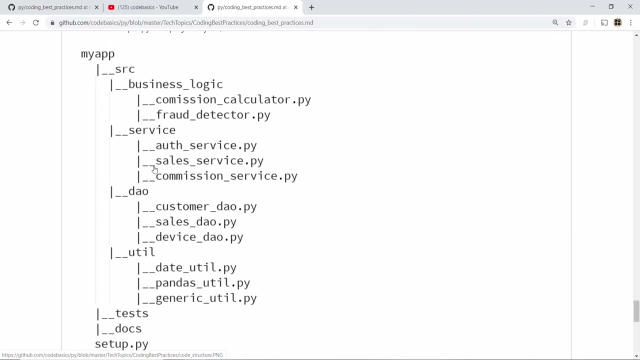 modify one function and all other callers will get benefit from it. another guideline is to use a right structure to layout your code. I have shown here a structure of a python program where a typical python program will have source and test and doc directory at the root level. it will also have setuppi. read me all those files and then within 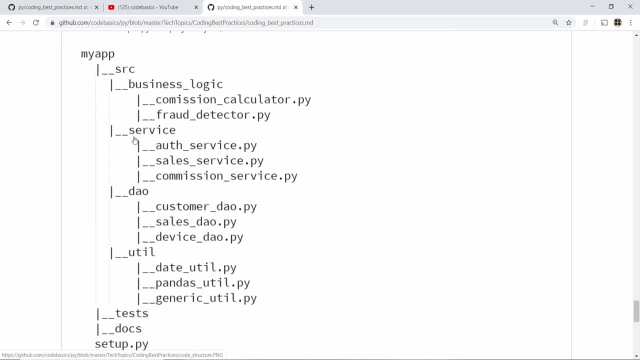 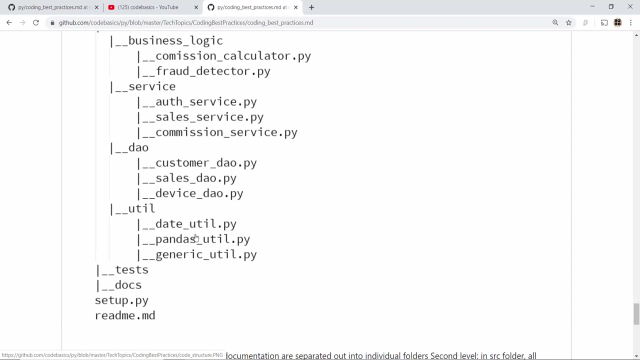 source. you can again organize your code by partitioning your files, uh, as per their purpose. for example, you could have service files, which is calling different services. you could have data access objects. you have utilities, for example you. you keep all your utility functions related to date and time. 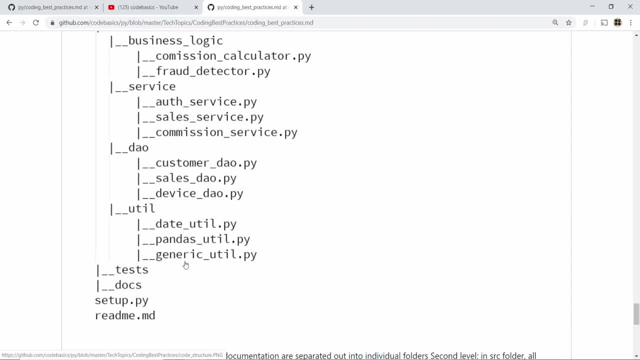 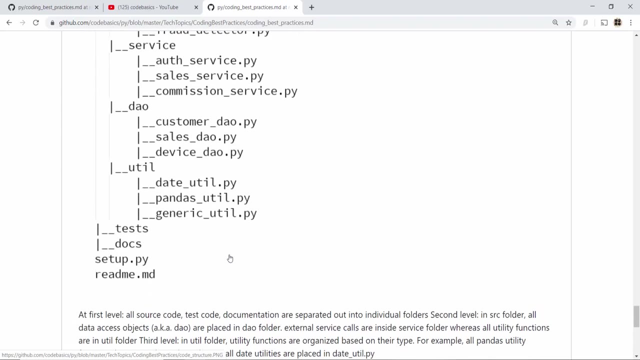 in data you tell if you are doing any pandas utility function. keep them in pandas util. so this way your code is organized properly. if someone is referring to this code, it becomes very, very easy for that person to navigate through this code base. so using a right structure is important also. 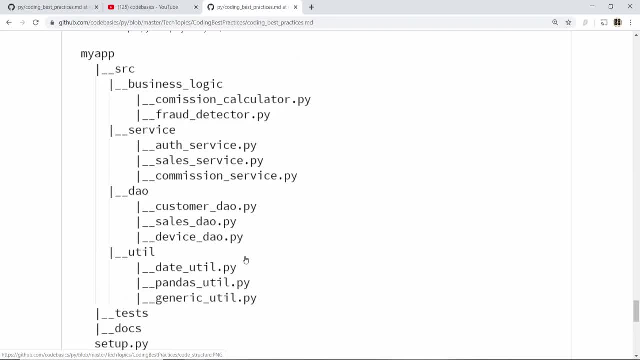 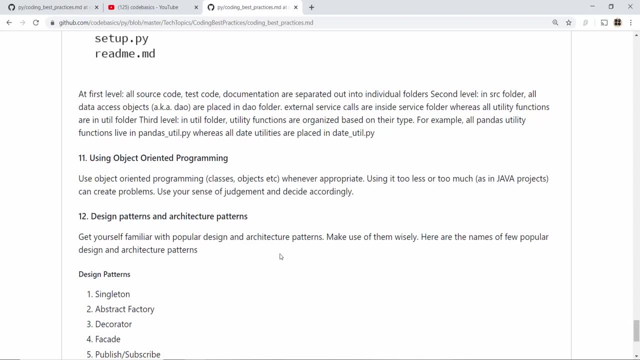 don't write all of your code in one file. try to organize your code in multiple files. using object oriented programming is also important. do not over use it or do not under use it. I mean that's that's the guideline here. I've seen some Java code bases. 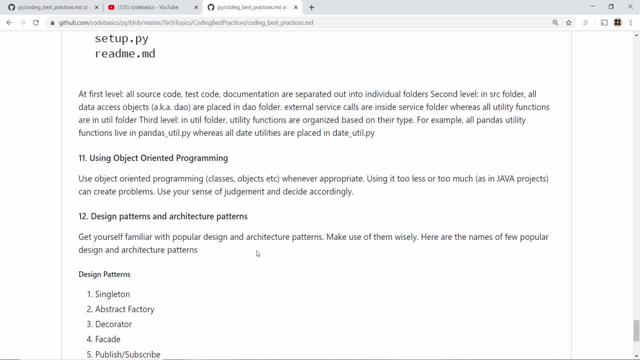 where they just overuse object oriented programming. they end up creating classes for pretty much everything, and that's not good. on the other hand, you don't want to have a single function which is, let's say, thousand line of code, because there's just too too many lines. you don't want to have too 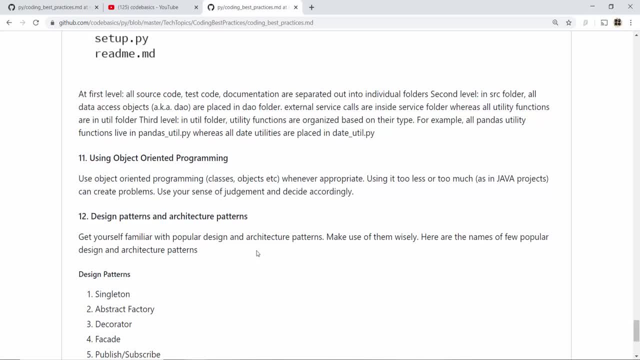 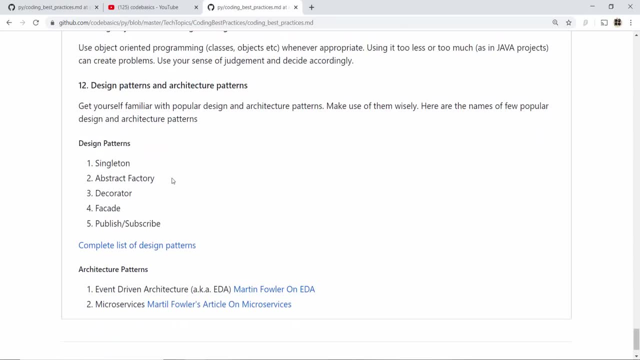 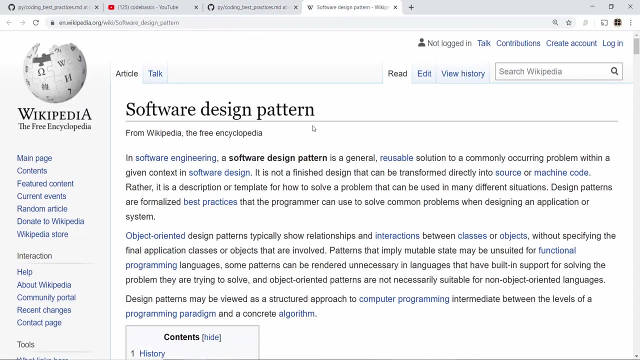 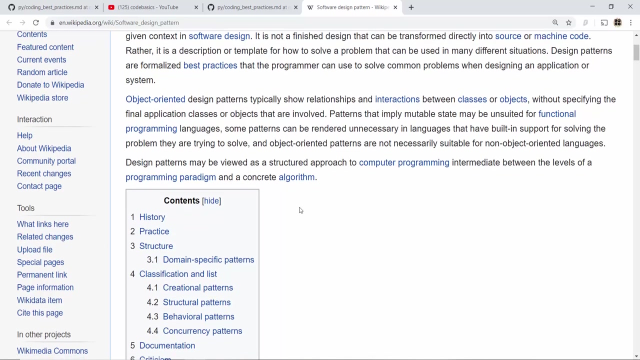 many lines, you want to divide that code into smaller and smaller function. so use object oriented programming wisely and in a balanced way. another guideline is to use design pattern and architecture patterns. you can read all the design patterns here in this nice Wikipedia article that we have and try to use appropriate design pattern for a given problem. you can also use different architecture. 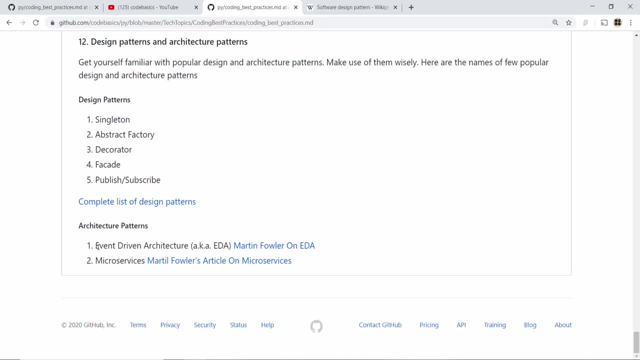 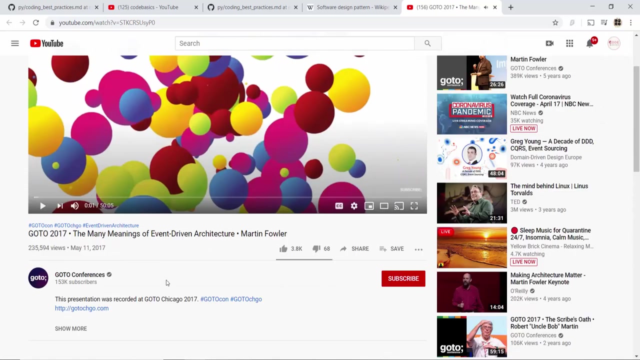 patterns and I have given few examples, such as event-driven architecture, also known as EDA or microservices for event-driven architecture. Martin Fowler has a great talk on what is event-driven programming. okay, so he presented this and go to conference in 2017. I'm gonna. 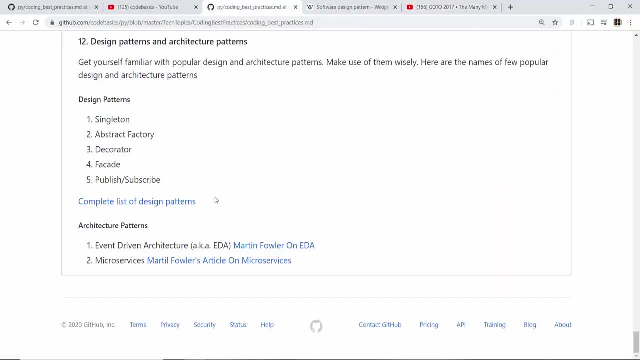 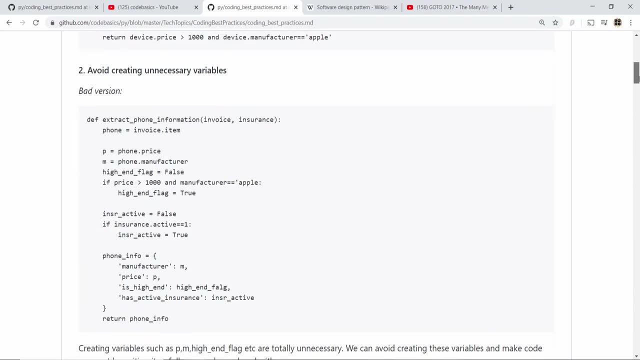 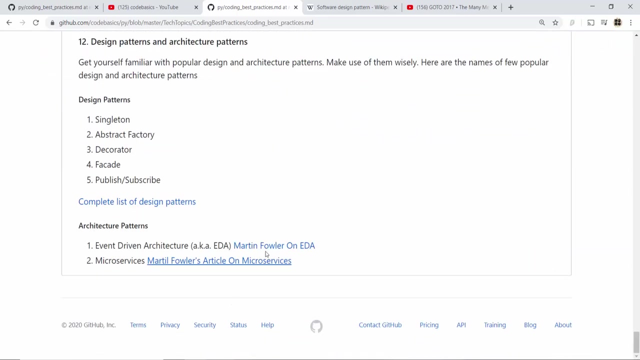 provide link of all this. okay, I have. by the way, I have made all these guidelines into a GitHub page so you can see that whatever we went through, they are available in this page, and I'm going to provide the link of this page in the video description. so this has a link of Martin Fowler's uh talk on. 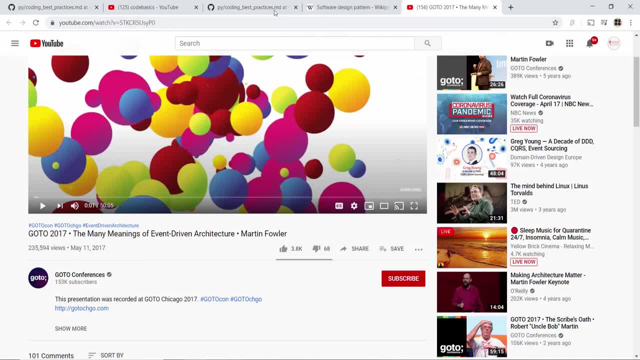 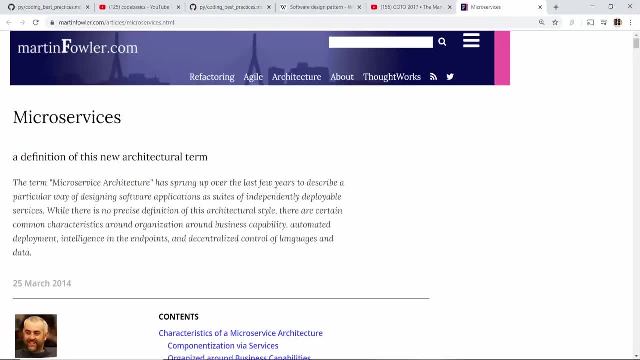 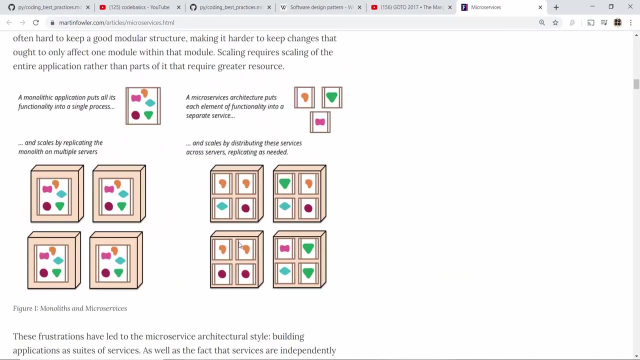 YouTube on event-driven architecture, so go through it. it's a very, very good talk. you can also use microservices instead of monolith. uh, so for microservices, my again. Martin Fowler has a great article here and it describes what is really microservices and how it can really help you. 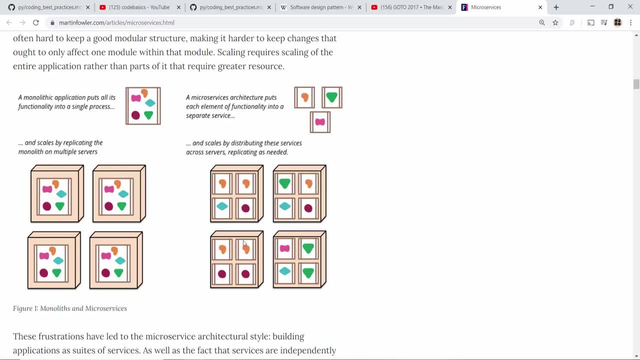 now you don't want to use microservice in all possible cases. I'm seeing that nowadays everyone microservice is a buzzword, everyone wants to move towards microservice. but you should really do microservices. uh, only if it is applicable to the problem that you are trying to solve. I attended 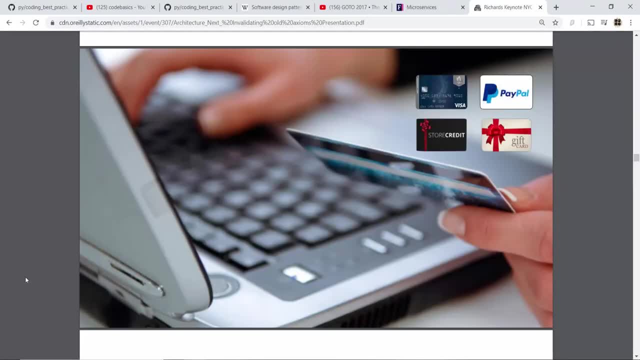 a software architecture conference recently in New York and Mark Richards gave a nice talk on when you should use microservice versus monolith. he gave example of a payment system. so, for example, let's say you are building a payment system which accepts payment from Visa card or PayPal or store credit or gift cards. now you can design your. 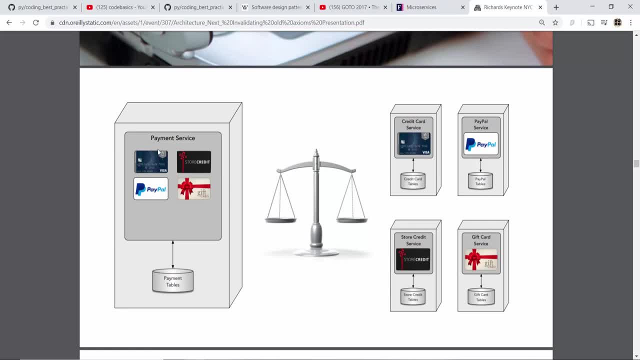 system in one of the two ways. on the left hand side is a monolith, so monolith service is a big service, accepts all kind of payments. on the right hand side I have microservice architecture where for each of the payment type I have a different microservice. now these microservices could be written in. 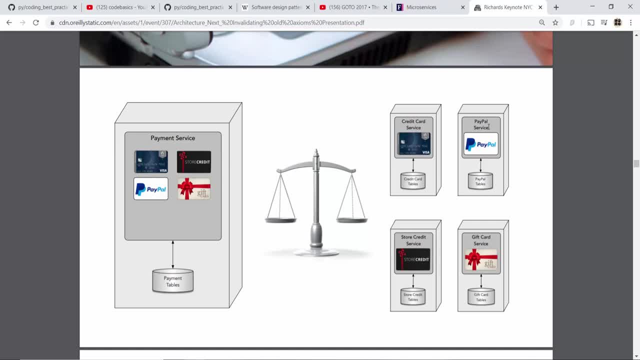 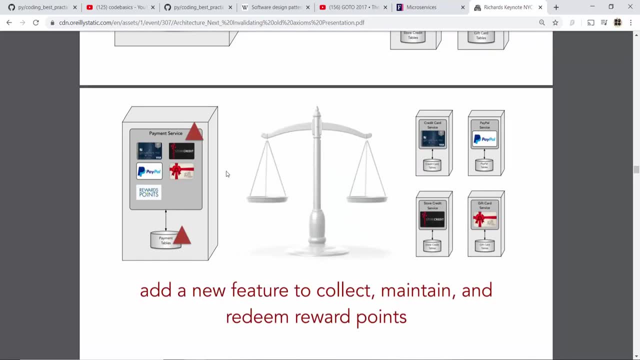 different programming language. for example, credit card service could be python, PayPal could be in Java. they could be owned by different teams as well. let's say you want to add a new feature to collect, maintain and redeem reward points on the left hand side in monolith architecture. when I add: 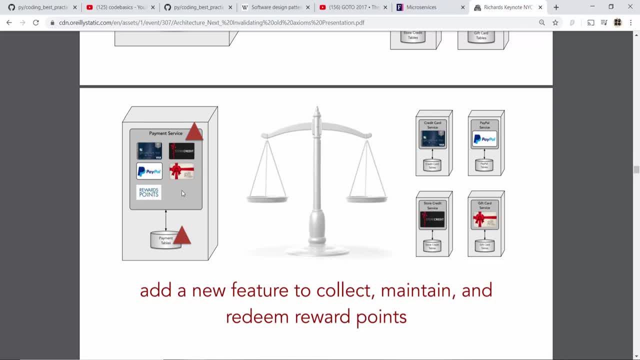 points code in this monolith. the issue that happens is I'm touching now this big code base. it might break some of the functionality with the remaining four components. the CI CD pipeline is affected and, um, you know it, it's. you're touching this big code base, so it could have. 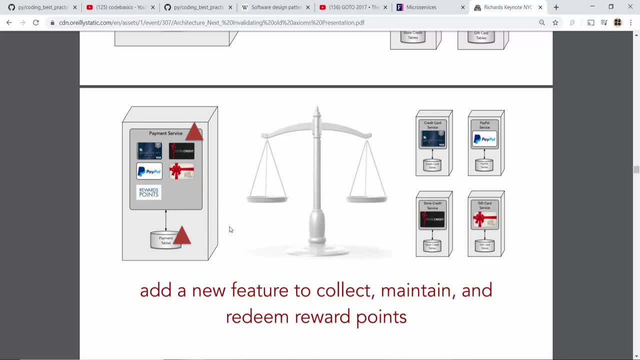 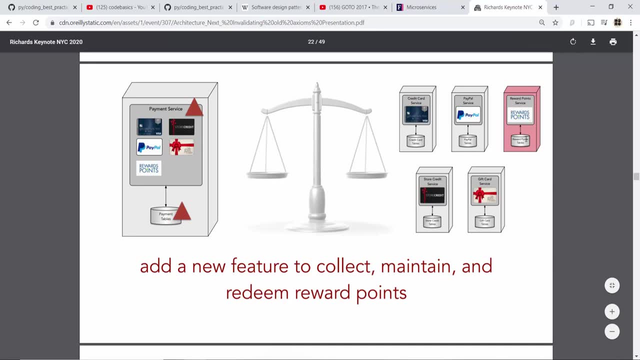 some implications that you don't want. on the other hand side, if you are using microservice architecture, what you are doing is creating a new component and now you are not touching the code for these four different pieces and they will continue to function as it is there. there is no, not a single. 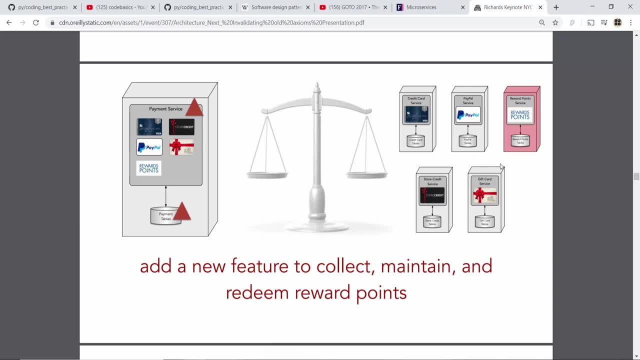 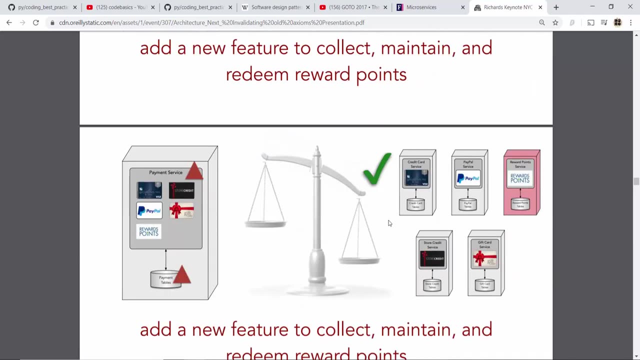 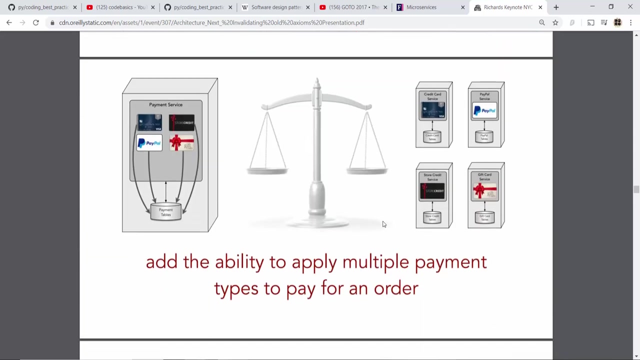 chance of having bugs in these four services, so also this service could be developed by a different team if these four teams are busy. so this way, if the components are running in isolation, and overall it becomes much, much easier. so in. so here, uh, microservice architecture wins. now let's say you. 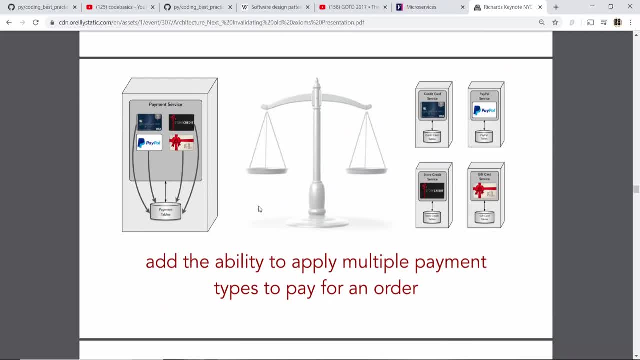 want to add the ability to apply multiple payment types for an order. let's say, customer puts hundred dollar order, seventy dollar you want to get from credit card and thirty dollar you want to get from PayPal. in this particular case, if it is in a same code base, it becomes much easier. so here, monolith. 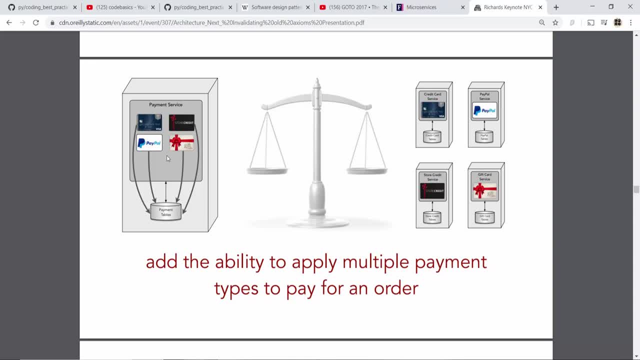 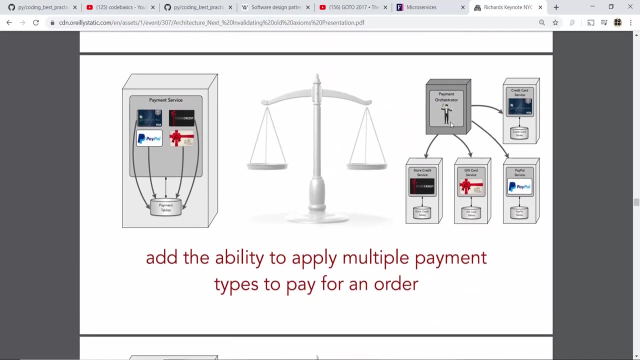 taking seventy dollar from credit card, thirty dollar from PayPal. it's in the same code base. you can use the functions of these different components and you know it's overall easier to manage. in case of my microservice architecture, you will have to create a payment orchestrator which will orchestrate. 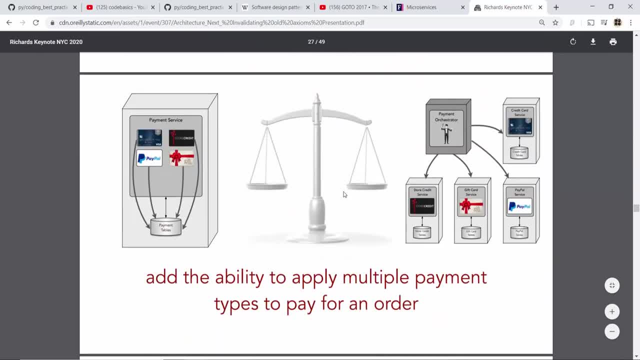 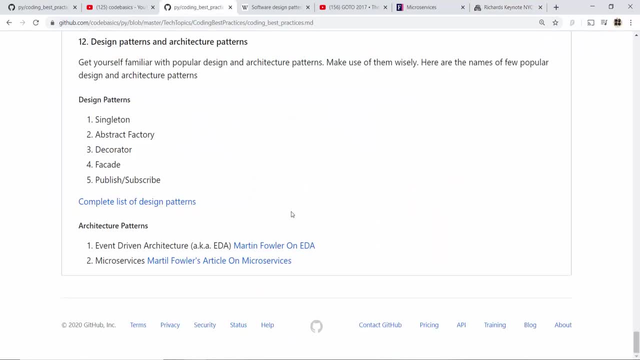 these different payments and it becomes really uh tough to manage. so here, uh, having monolith wins. one exercise, which is: if you are aware about any other coding practices which you feel is good which I have not covered, please post in a video comment below. thank you.